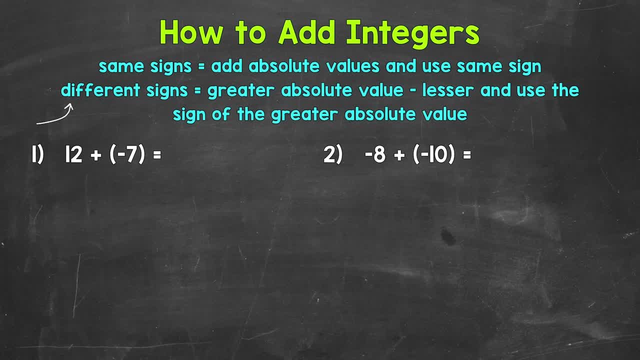 Since we have different signs, we are going to take the greater absolute value and subtract the lesser. Our answer will take the sign of the greater absolute value. let's start by writing the absolute value of both 12 and negative 7.. And remember: 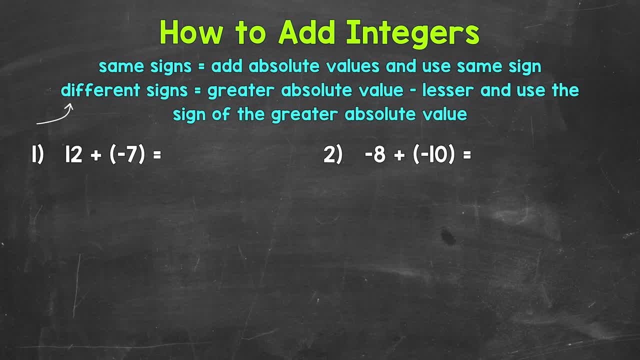 absolute value is the distance a number is from zero. The absolute value of 12 is 12.. The absolute value of negative 7 is 7.. Now we take the greater absolute value and subtract the lesser. These are all the signs that we have. We're going to start by writing the absolute value. 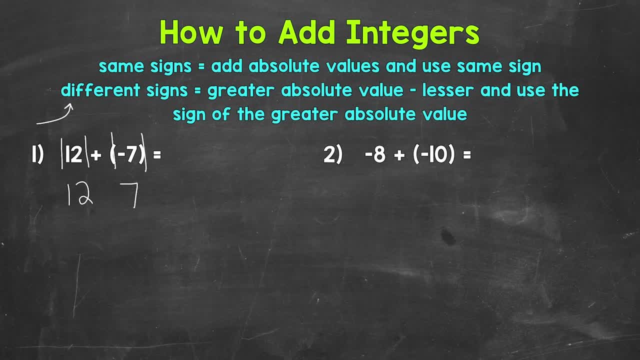 already in order, so we can subtract If the larger absolute value comes second. you can always switch the order to find the difference, if need be. Let's subtract. So 12 minus 7 is 5.. Now we need to determine if our answer is going to be positive or negative. 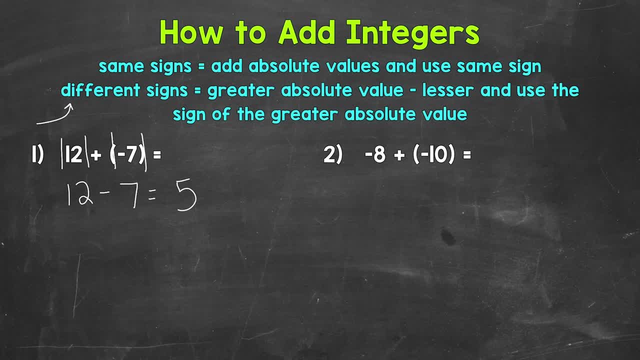 So we need to take a look at the larger absolute value, which is this 12.. Let's take the sign of the larger absolute value from the original problem. So the larger absolute value is 12.. Let's take a look at the 12 in the original problem. 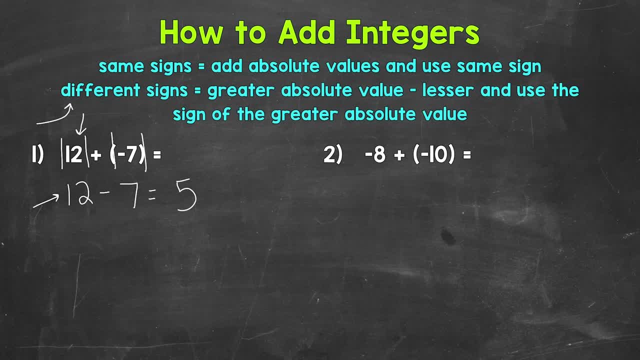 And that 12 is positive, That means our answer is going to be positive. So our final answer: a positive 5.. So a quick recap here. Basically, we forgot about any negatives because we were working with absolute values. We then found the 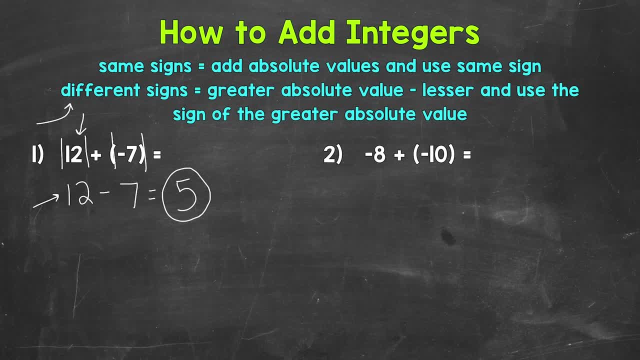 difference between the absolute values, and the answer takes the sign of the greater absolute value from the original problem. Now let's think through this another way, And this way is going to be more of a mental math approach, Just basically thinking about what's going on in. 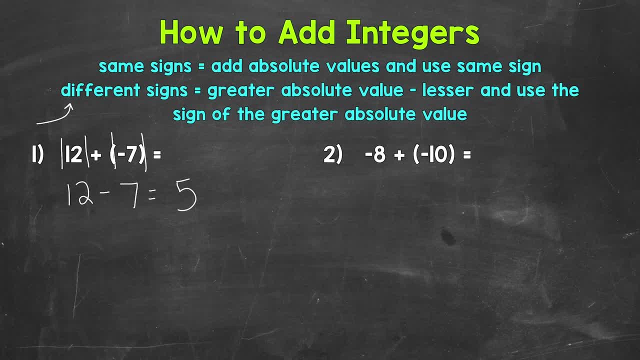 So we need to take a look at the larger absolute value, which is this: 12.. The larger absolute value is 12.. We need to take a look at the 12 in the original problem and that 12 is positive, That means our answer is going to be positive. So our final answer: 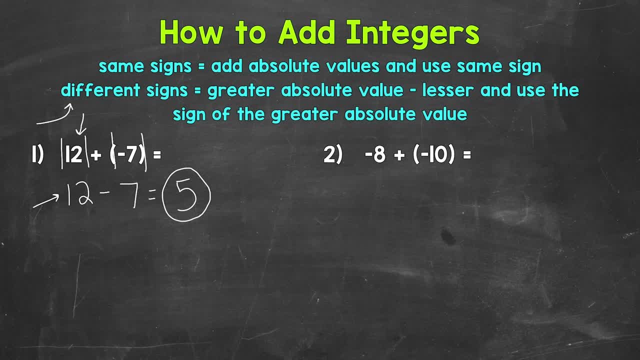 a positive 5.. So a quick recap here. Basically, we forgot about any negatives because we were working with absolute values. We then found the difference between the larger absolute value and the larger absolute value, So we're going to take the sign of the larger absolute value from the. 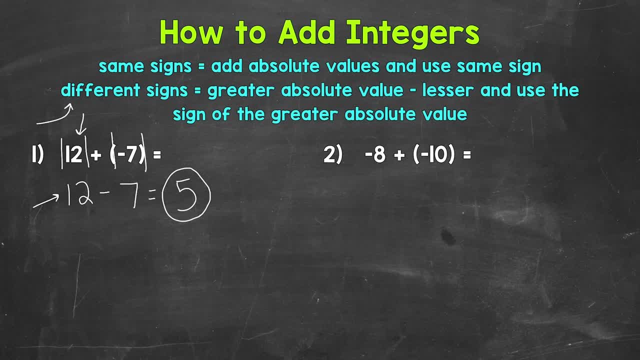 difference between the absolute values, and the answer takes the sign of the greater absolute value from the original problem. Now let's think through this another way, And this way is going to be more of a mental math approach, Just basically thinking about what's going on in this problem. So let me 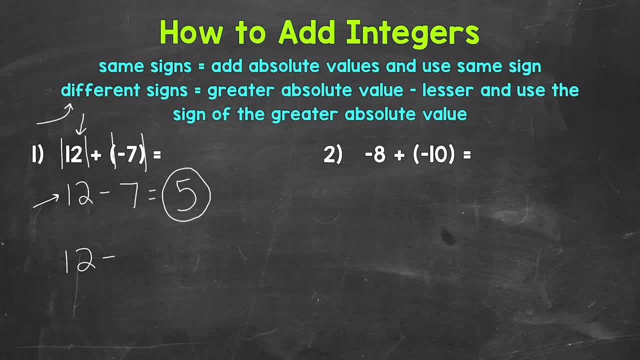 rewrite 12 plus negative 7 here. So our original problem is going to be positive. So we're going to our original problem. So we are starting at a positive 12, and we are adding a negative 7.. By adding a negative, by adding that negative 7, we are decreasing in value by 7 from that 12.. We can. 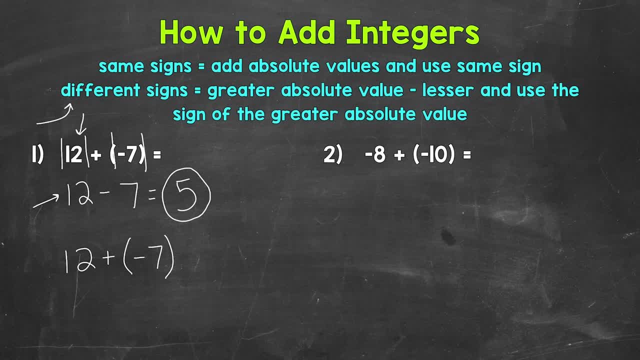 basically think of this as 12 minus 7 or 12 take away 7. That gives us our answer of 5.. So 12 plus negative 7. We are decreasing that 12.. We are decreasing that negative 7. We are decreasing that. 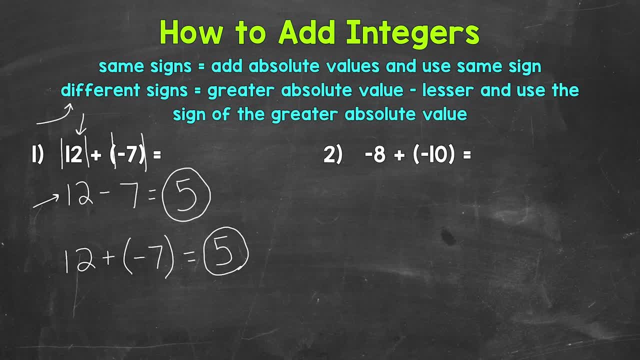 12 by a value of 7.. So we get a positive 5.. So again we started at a positive 12.. Always think about where you are starting and where you are going from that starting point. So we are adding a negative 7,, which is decreasing our 12 in value by 7, and we end up with 5.. Let's move on to number. 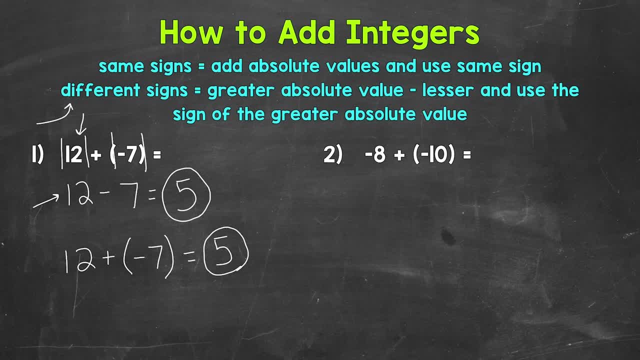 2, where we have negative 8 plus negative 10.. Here we have two negatives, so the same signs. So we are going to add the absolute values and use the same sign. So let's start by taking a look at the absolute value of negative 8 and negative 10.. The absolute value of negative 8 is 8.. 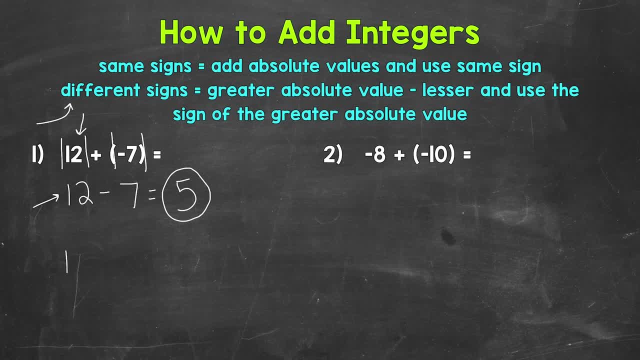 this problem. So let me rewrite 12 plus negative 7 here. So our original problem. So we are starting at a positive 12 and we are adding a negative 7.. By adding a negative, by adding that negative 7, we are decreasing in value by 7 from that 12.. We can basically think of this as 12 minus 7,. 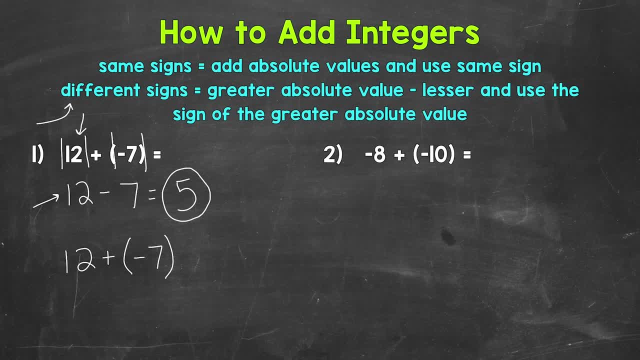 or 12-7.. take away 7, that gives us our answer of 5, so 12 plus negative 7. we are decreasing that 12 by a value of 7, so we get a positive 5. so again we started at a positive 12. always think about. 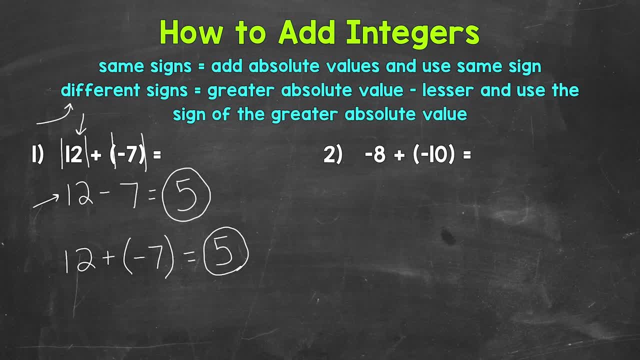 where you are starting and where you are going from that starting point. so we are adding a negative 7, which is decreasing our 12 in value by 7, and we end up with 5. let's move on to number 2, where we have negative 8 plus negative 10. here we have two negatives, so the same signs. 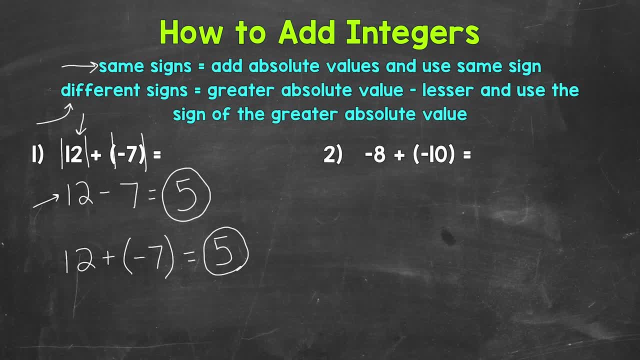 so we're going to add the absolute values and use the same sign. so let's start by taking a look at the absolute value of negative 8 and negative 10. the absolute value of negative 8 is 8 plus the absolute value of negative 10, which is 10. now we add those. 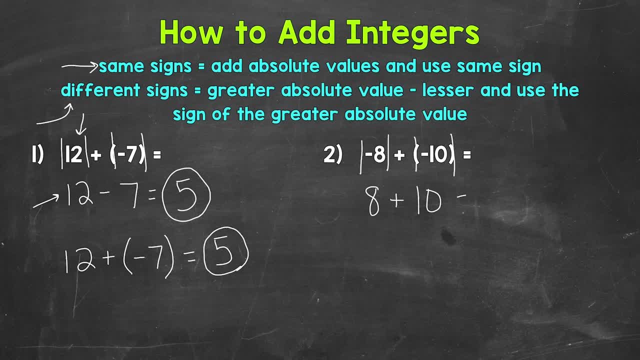 absolute values because again we have the same signs: 8 plus 10 is 18. we use the same sign from the original problem, which those are negatives there. so our answer is negative. final answer: negative 18. now if we were to think through this, we can think that we are starting at negative 8. 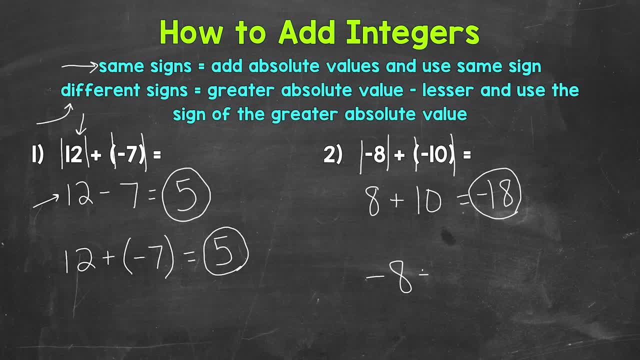 so let me rewrite here: negative 8 plus negative 10, so again starting at negative 8, and we are adding a negative 10. so that means we are decreasing in value by 10. that leaves us at negative 18, like i mentioned earlier. think about your starting point, so the number you. 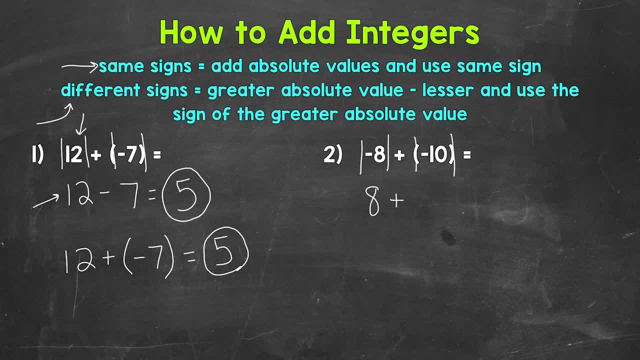 plus the absolute value of negative 10,, which is 10.. Now we add those absolute values because again we need to go back to our. we had the same signs: 8 plus 10 is 18.. We use the same sign from the original problem, which. 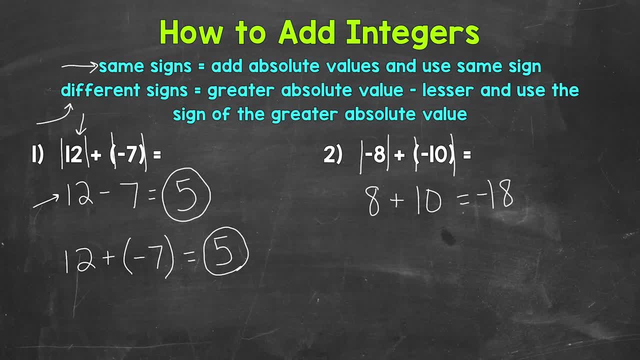 those are negatives there. so our answer is negative. Final answer: negative 18.. Now if we were to think through this, we can think that we are starting at negative 8.. So let me rewrite here: negative 8 plus negative 10.. So again starting at negative 8, and we are adding a negative 10.. 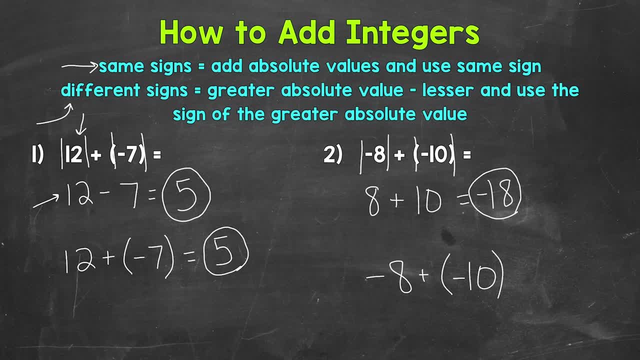 So that means we are decreasing in value by 10.. That leaves us at negative 18.. Like I mentioned earlier, think about your starting point. so the number you are starting with, We have a negative 8, and then adding that negative 10 tells us we are decreasing in value and end up. 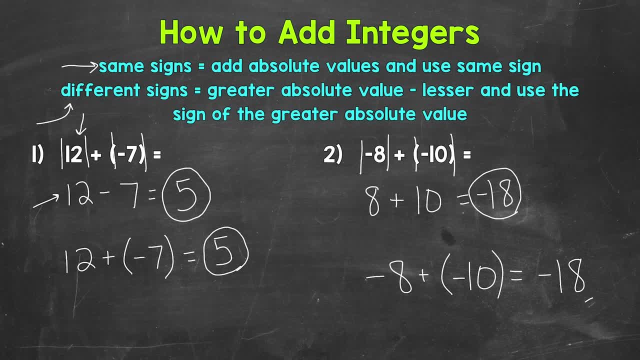 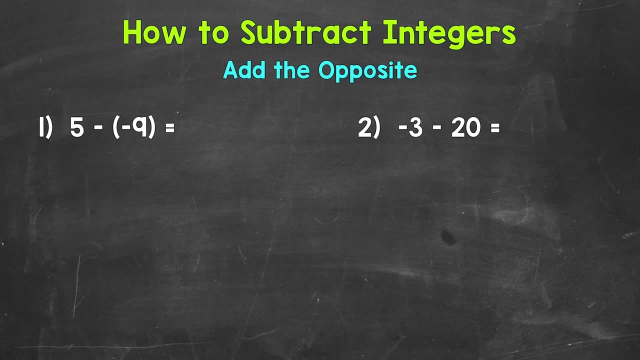 negative 18.. Negative 18 is our final answer. That's how we add integers. Let's move on to subtraction. So here are our examples for subtracting integers. Let's jump into number 1, where we have 5 minus negative 9.. Now, when we subtract integers, we're actually going to 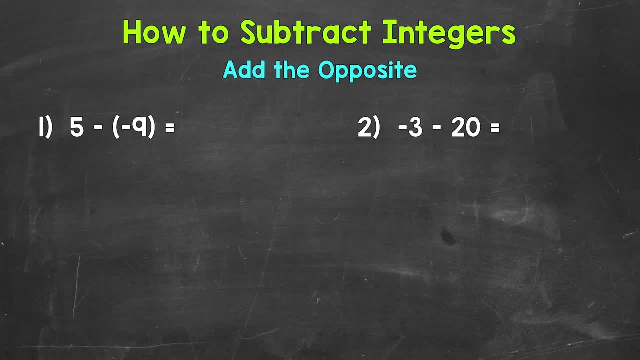 add the opposite. So if you're able to add integers, you're going to be able to subtract integers. The opposite of subtraction is addition, And then we take the opposite of the number we are subtracting. So this gives us an equivalent problem and we are able to use this strategy. 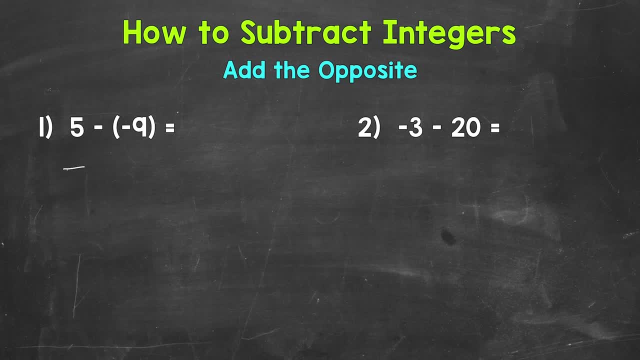 So we have 5, and then let's add the opposite of negative 9.. The opposite of negative: 9 is positive 9.. So 5 minus negative 9 is positive 9.. So 5 minus negative 9 is positive 9.. So 5 minus. 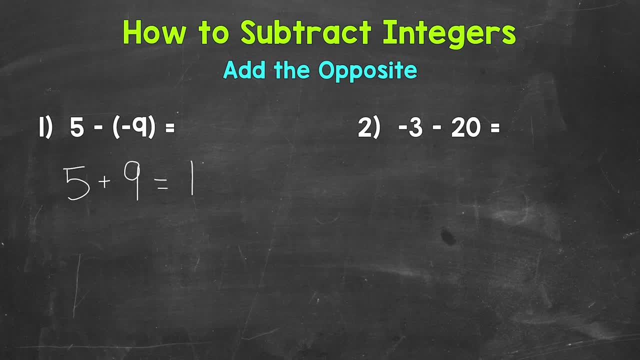 negative 9 is positive 9.. So 5 plus 9, that gives us 14, a positive 14.. And that's our final answer. Now, that answer may not make sense at first, but let's think about how we end up with a positive. 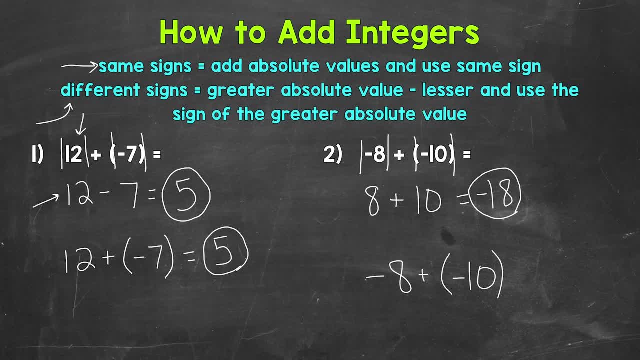 are starting with is negative 8 and we are adding a negative 10. so that means we are starting with we have a negative 8 and then adding that negative 10 tells us we are decreasing in value and end up at negative 18. negative 18 is our final answer. that's how we add integers. let's move. 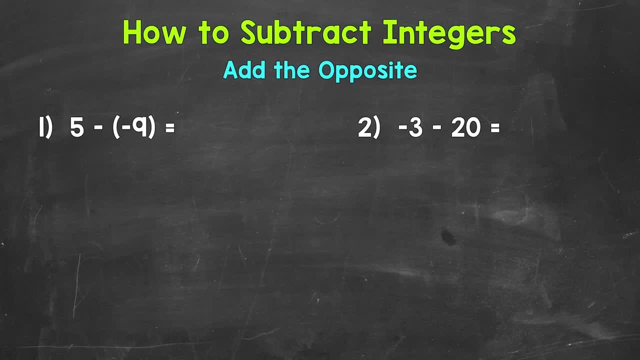 on to subtraction. so here are our examples for subtracting integers. let's jump into number one, where we have 5 minus negative 9. now, when we subtract integers, we're actually going to add the opposite. so if you're able to add integers, you're going to be able to subtract. the opposite of subtraction is addition. and then we 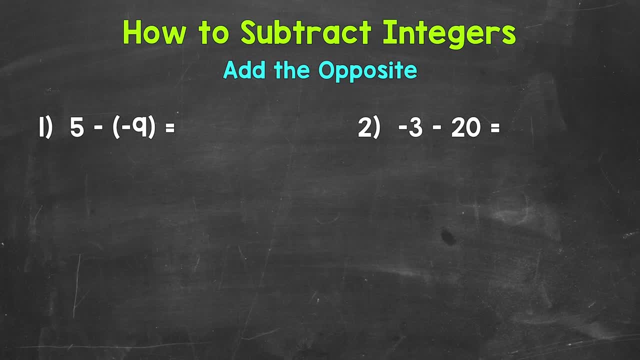 take the opposite of the number we are subtracting. so this gives us an equivalent problem and we are able to use this strategy. so we have 5. and then let's add the opposite of negative 9. the opposite of negative 9 is positive 9. so 5 plus 9, that gives us. 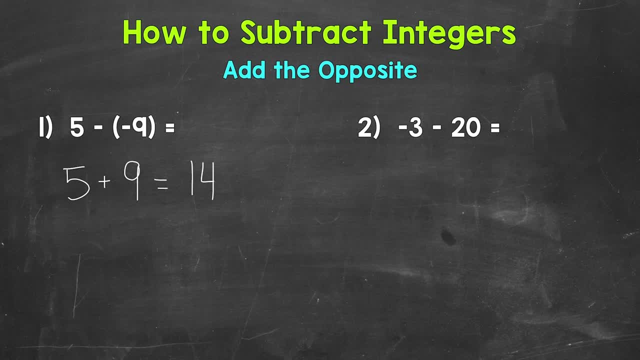 14, a positive 14, and that's our final answer. now that answer may not make sense at first, but let's think about how we end up with a positive 14 in this subtraction problem. whenever we subtract a negative, we actually increase in value. i like to think of this in terms of money. a negative 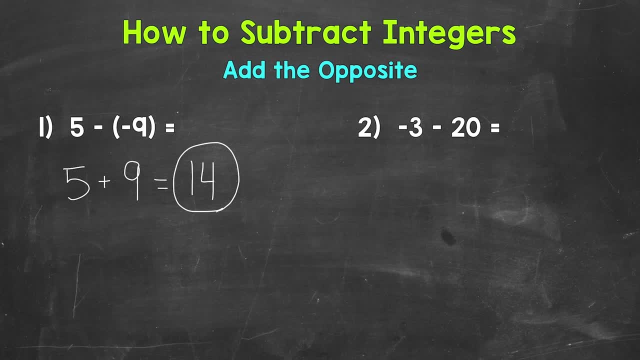 represents a debt or an expense when it comes to money. so that negative 9 would be a nine dollar debt or expense. think of subtracting a negative, like subtracting or taking away that debt or expense and getting that money back. that is a good positive 9. so let's think about how we end up with a. 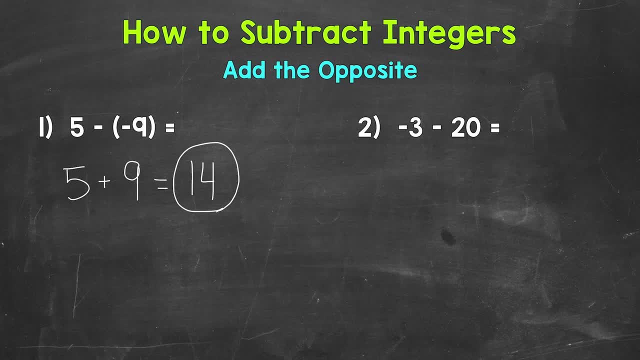 negative 14 and add 5. in the same way, a negative 10 is good. so what we're going to do is we're going, we're going to go back and look at both two things. so i'm going to go back to minus 14 and add a. 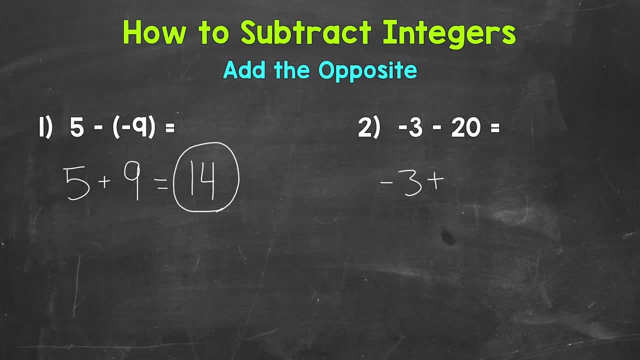 minus 4 for the last time, okay, and i'm going to go ahead and add a add something for other three. so what we're going to do now is we are going to go over to minus 7 and we're going to subtract a negative 15 plus. that was a lot of 천ente.